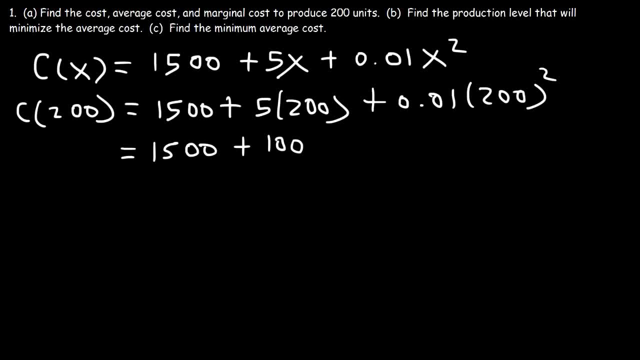 Now 5 times 200, that's 1000.. And 200 squared is 43.. So 1500 plus 1000 times 0.01, that's going to be 400.. So 1500 plus 1000, that's 2500 plus 400, so that's 2900.. 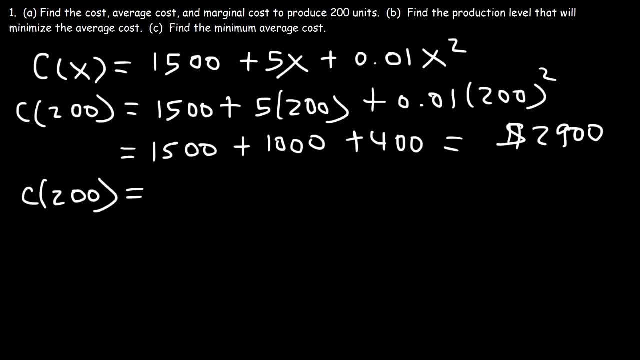 So the production level at 200, so that is, the total cost of selling 200 units- is $2900.. Now what about the average cost? Let me write that down, All right, per 200 units. So what's the average cost per unit? 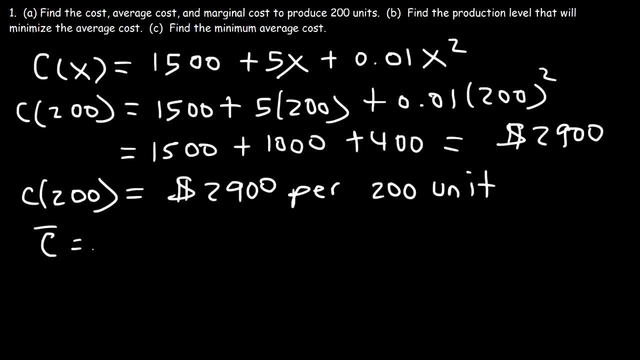 The average cost is basically the cost divided by x, So it's going to be 2900, the total cost to make 200 units divided by those 200 units, And so we could cancel the two zeros, and then it becomes 29 divided by 2,. 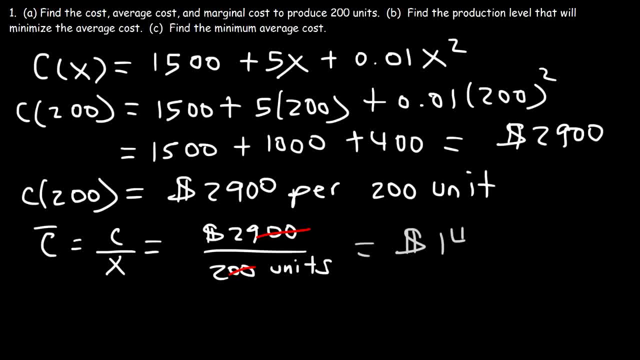 which is $14.50.. So that's the average cost to make one unit of an item. Now what about the marginal cost? How can we determine the marginal cost to produce 200 units? Let's see The marginal cost. The marginal cost. 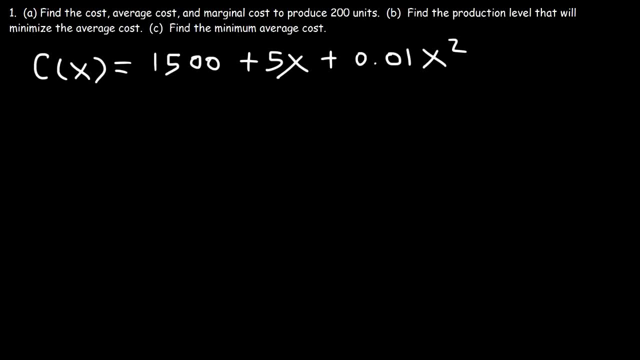 Is basically the first derivative of the cost function, So it's C prime of x. The derivative of a constant like 1500, is 0.. The derivative of 5x is 5.. And the derivative of x squared is 2x times 0.01.. 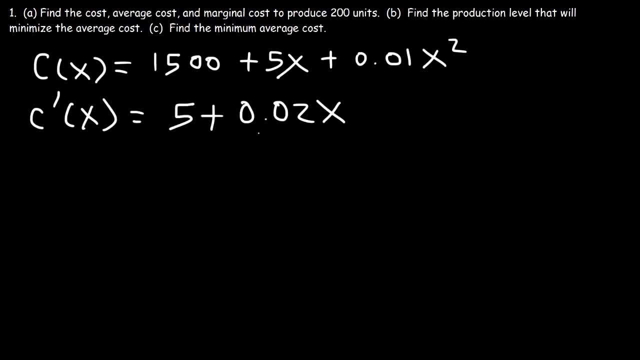 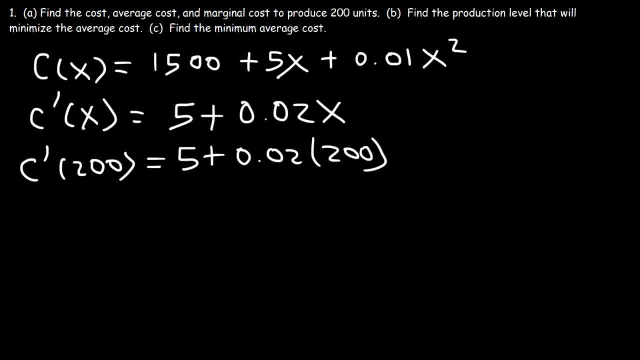 So that's 0.02x, So that's 0.02x, So that's 0.02x. Now, 2 times 200 is 400.. 0.2 times 200 will be 40. So 0.02 times 200 is 4.. 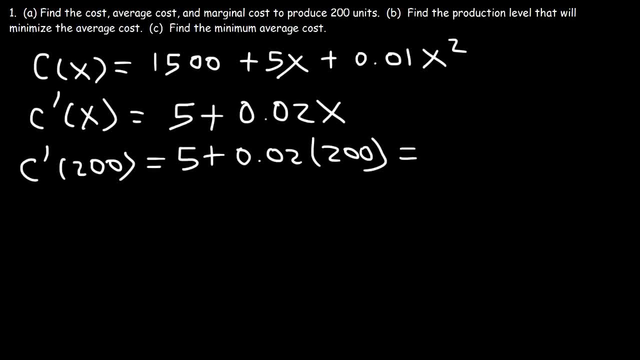 And then 4 plus 5 is 9.. So this is basically $9 per unit. So what does this tell us? What's the basic idea behind the marginal cost? The marginal cost tells us the additional cost is the number of units that are produced. 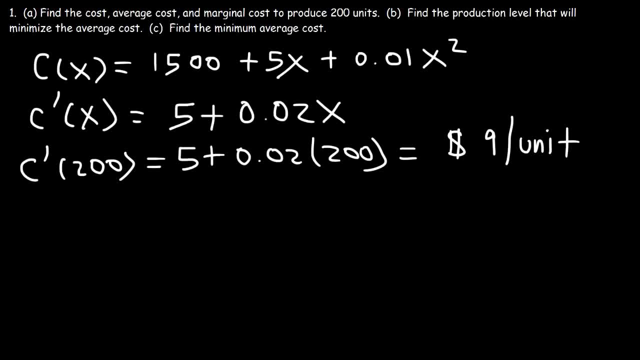 costs that it will take to make one extra unit. So we said that the total cost to make 200 units, if you recall, was $2900.. So what is the total cost to make just one extra unit? So 1 plus 200 is 201.. 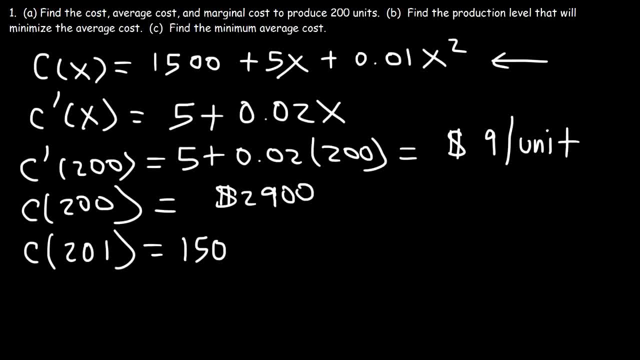 Well, let's plug it into this equation and let's see what's going to happen. So it's 1500 plus 5 times 201, plus .01 times 201 squared, So this is still going to be 1500.. Now, 5 times 200 is 1000, and 5 times 1 is 5.. 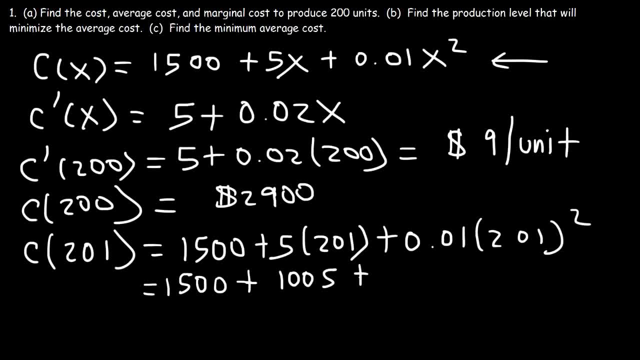 So that's going to be 1005.. And then 201 squared times .01.. That's 404.01.. Okay, So let's go ahead and add the three numbers, So this will give you 2909.01.. Now look at the difference between the cost at a production level of 200 and the total. 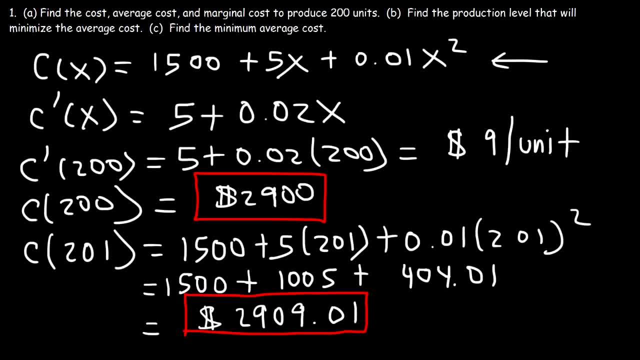 cost at a production level of 201.. The difference between those numbers, if you take 2909.01 and subtract it by 2, that's $2900.. So that will give you a difference of $9.01.. So the cost to make an additional unit increased by $9 approximately. 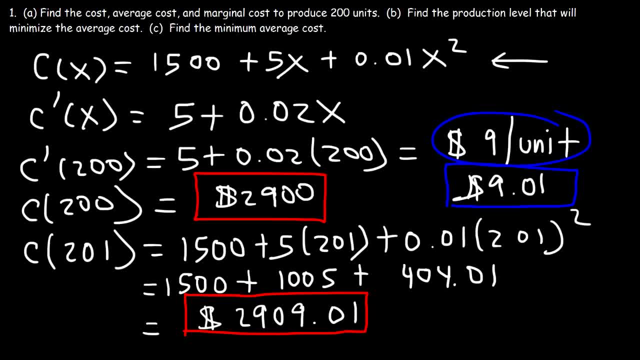 And that's what the marginal cost tells us. It tells us how much it will cost us if we're going to produce one extra item, And you can see that based on the difference between the cost Between these two values. Now let's move on to Part B: Find the production level that will minimize the average cost. 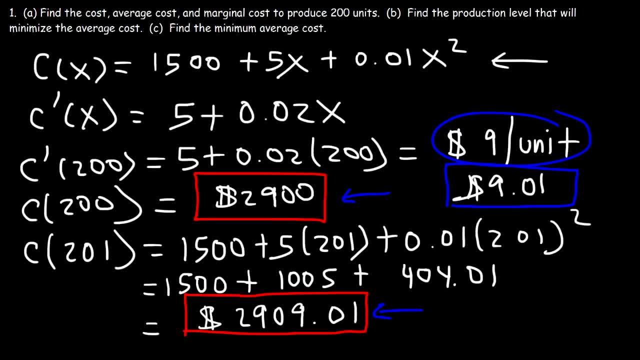 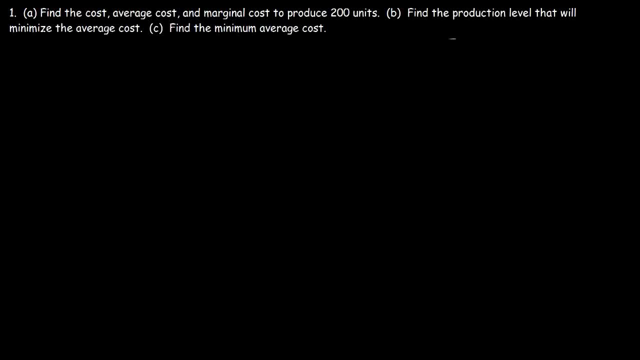 So how can we do that? In order to find the minimum average cost, or the production level that leads to the minimum average cost, you need to know a simple fact, And that is that the average cost is a minimum cost. This is a minimum when the marginal cost is equal to the average cost. 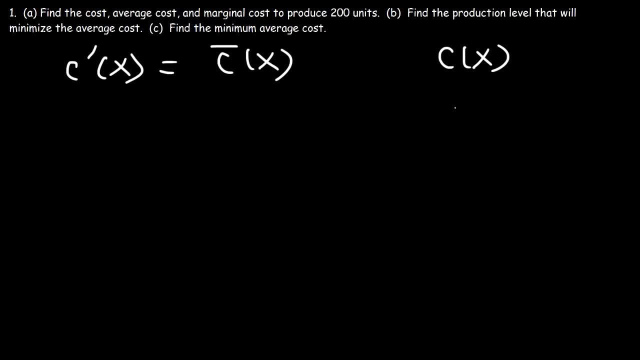 By the way, C of X, I'm going to use that to represent the total cost function. And when you see this line above the C, I use that to represent the average cost function. Just in case you're wondering Now, we said the marginal cost was basically 5 plus .02x. 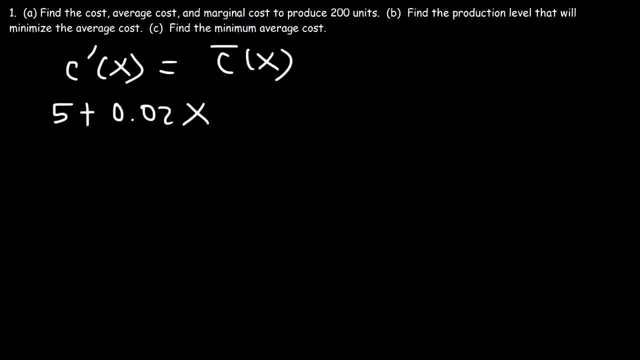 That's the average cost. That's the total cost. Now, the average cost is basically the cost function divided by X. Now, the cost function, which is what we had at the very beginning, That was 1500 plus 5x plus .01x squared. 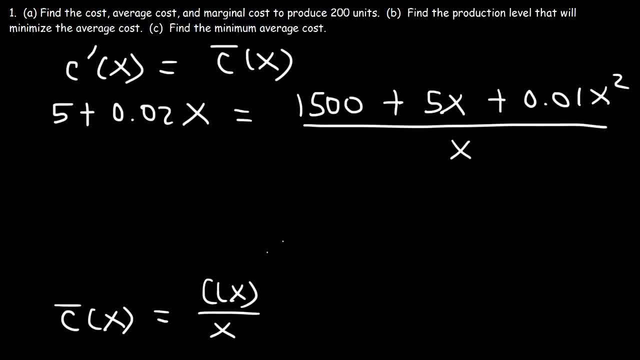 Now we need to divide this function by X, And then it becomes the average cost function. So I'm going to divide every term by X Separately, Which is the same as dividing the whole thing by X. So everything on the right side now represents the average cost function. 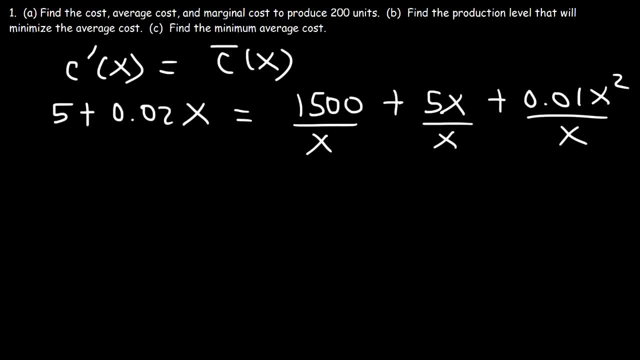 So all we need to do at this point is solve the equation. X represents the production level, So we need to calculate the value of X. The left side is going to stay the same for now, And on the right side We're going to have 1500 divided by X. 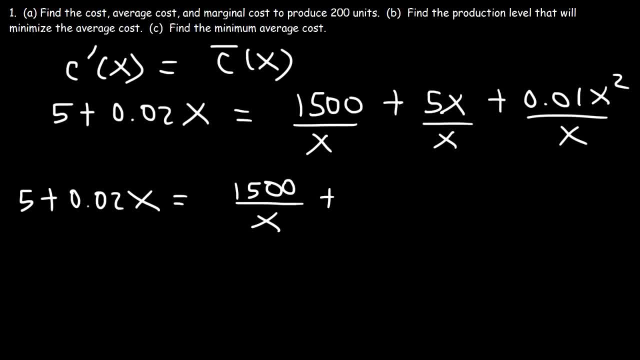 5x divided by X, The X variables will cancel, And so that's going to give us 5.. And X squared over X, That's just X. So we're going to have .01x Now if we subtract both sides by 5.. 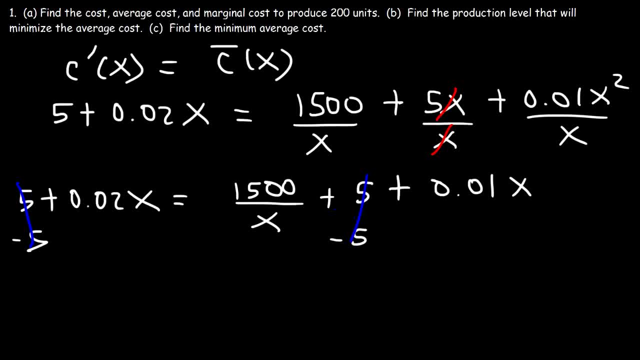 They will cancel. So that's just going to disappear. And then we need to subtract both sides by .01x. So on the right side these will cancel, And on the left .02 minus .01 is .01.. And that's equal to 1500 divided by X. 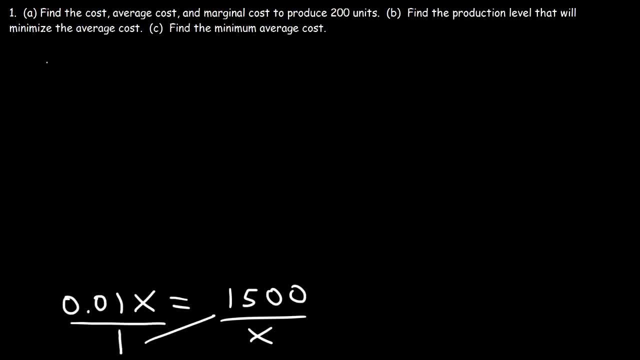 So now what we need to do is cross, multiply. 1500 times 1 is 1500.. And then .01x times X, That's .01 x squared. So let's divide both sides by .01.. 1500 divided by .01.. 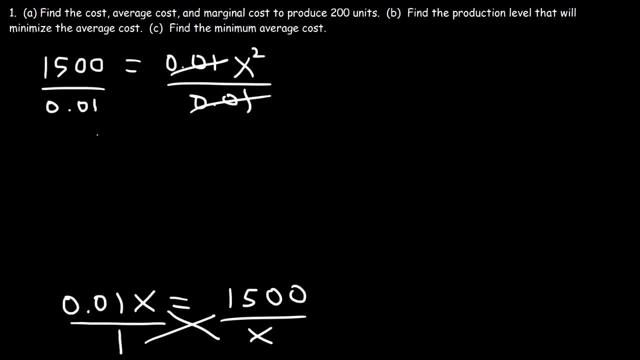 When you divide by .01, it's the same as multiplying by 100.. So this becomes 150000.. And that's equal to x squared. So now we need to take the square root of both sides, And so X is going to be 387.3,. but we need to round to the nearest unit. 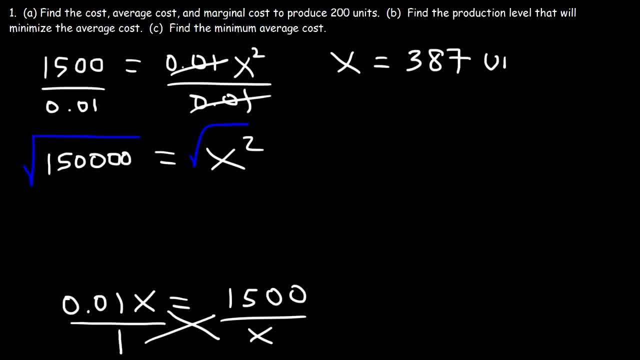 So we're going to say it's about 387 units. So that's the production level that will minimize the average cost. So at this production level the average cost should be the lowest value. Part C: we need to find the minimum average cost. 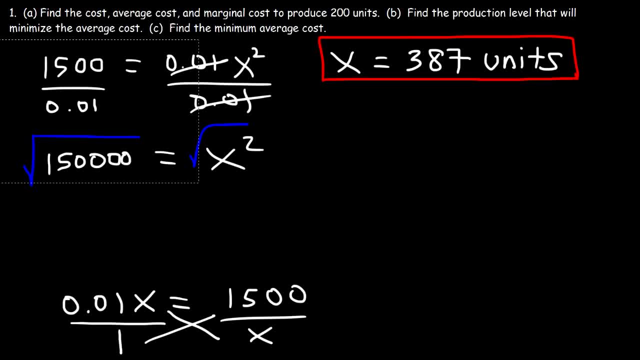 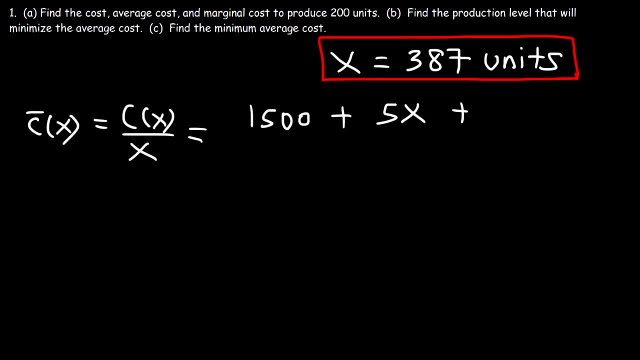 So we need to take this X value and plug it into the average cost function. Now we said that the average cost function is the total cost function divided by X. Now the total cost function was 1500.. This is the original problem that we had, or the original equation: plus 5X plus 0.01X squared. 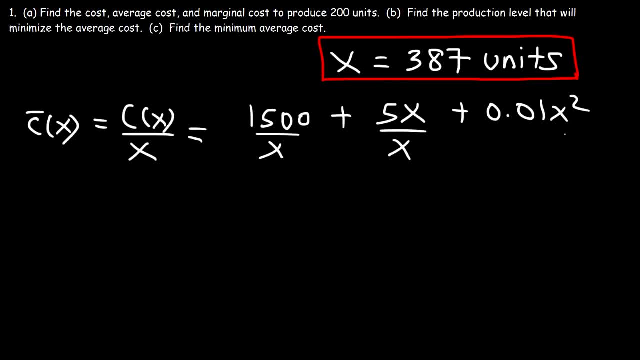 And to find the average cost you need to divide it by X. So the average cost function is 1500 over X plus 5 plus 0.01X. So let's calculate the average cost at 387 units. So let's see what answer we're going to get.